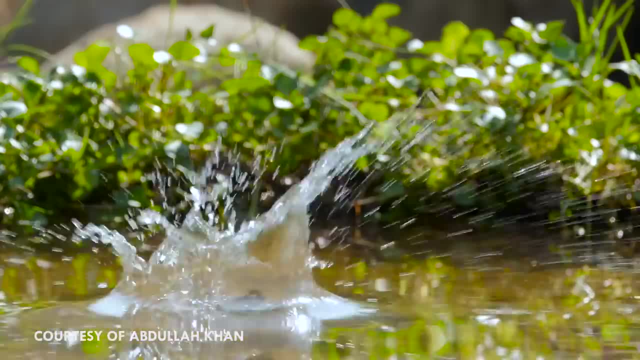 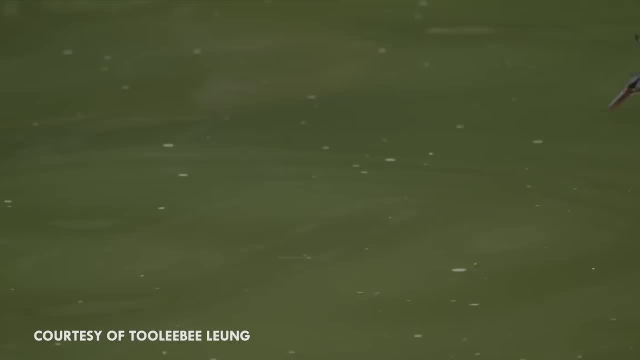 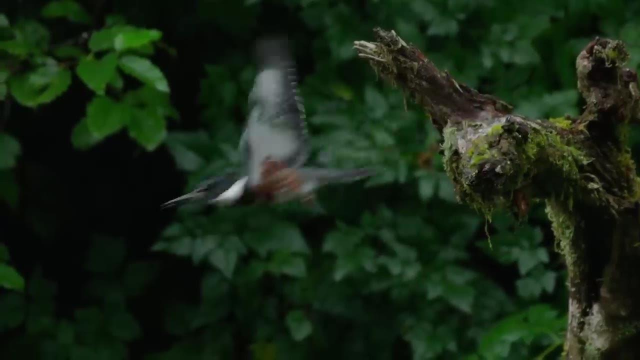 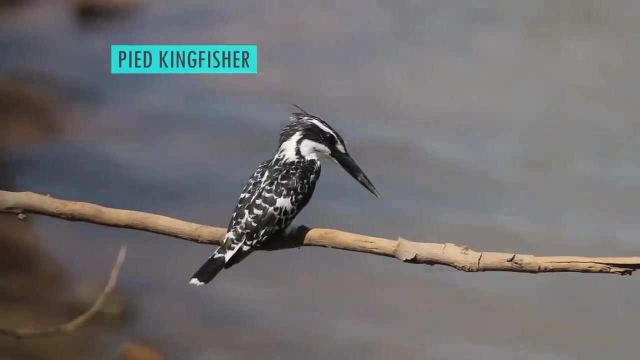 dive Kingfishers will perch on a branch overlooking the water and wait for the perfect opportunity to dive-bomb their prey. Some species of kingfisher take this to the next level, like the pied kingfisher, which is the largest bird in the world that can hover in place. They beat their way up to the top of the mountain. and then they dive to the top of the mountain with their wings- eight times a second, much like a hummingbird, only several times larger. Some species will hover up to 10 meters above the water. 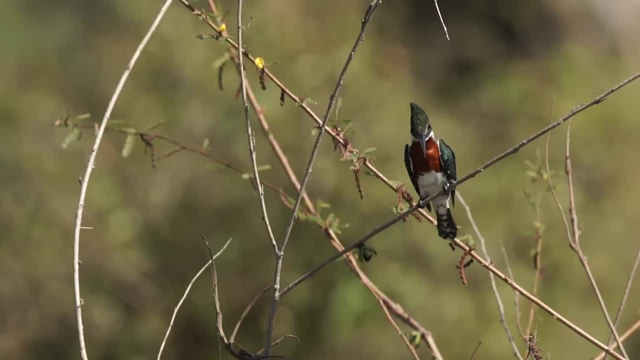 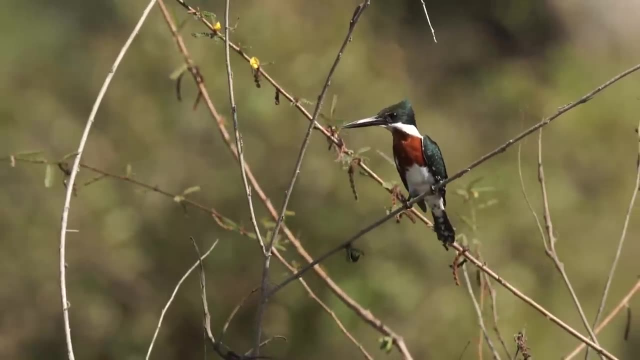 high enough to be sure that they won't be spotted by any would-be prey. Kingfishers have very strong and adept muscles in their neck which they use to keep their head stabilized while searching for fish. Like many other predatory birds, they have very large eyes. 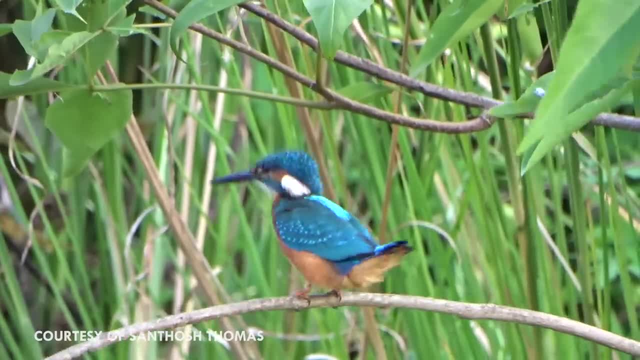 with a limited range of movement that give them an increased ability to pick out prey at a distance. They have an intense sense of smell and they're very capable of finding prey at a distance. They have an intense sense of smell and they're very capable of finding prey at a distance. They have an 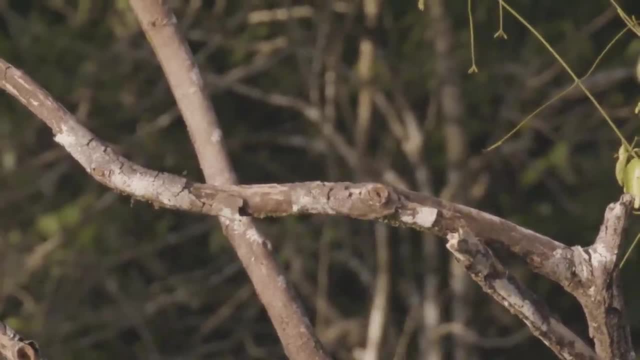 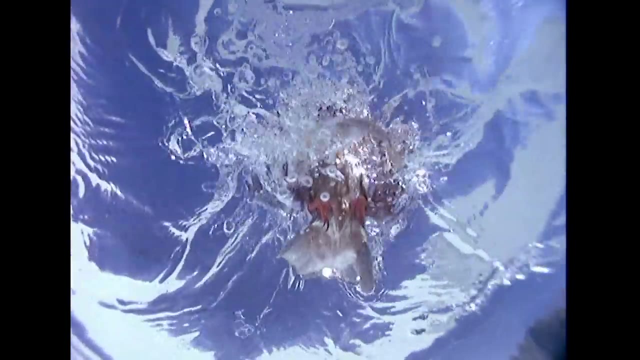 intuitive understanding of how water refracts light. taking that into consideration. as they dive down at full speed, Their beaks are shaped like needles and slide into the water with ease. When they hit the water, their prey has less than a second to react In order. 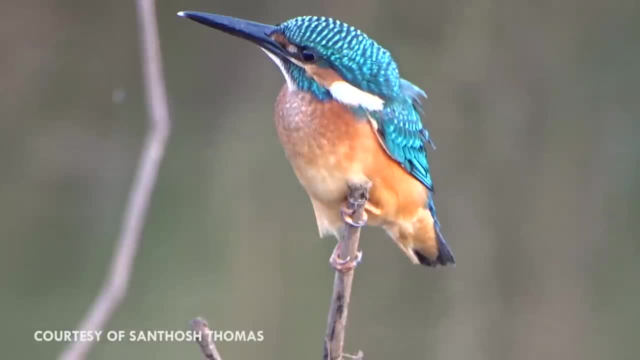 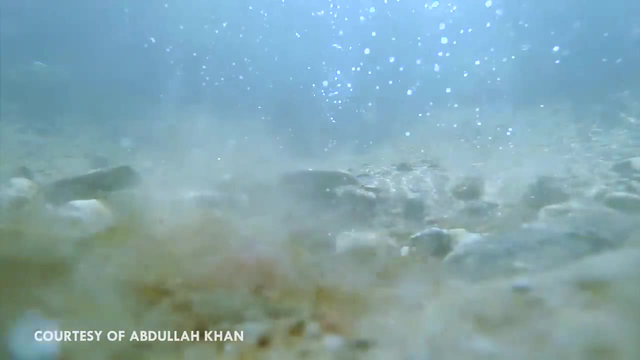 to keep track of where their prey is. their eyes have a third translucent eyelid called a nictitating membrane that protects their eyes from the water. This allows them to keep their eyes open while diving. If their prey is too large, they will hit it from above. 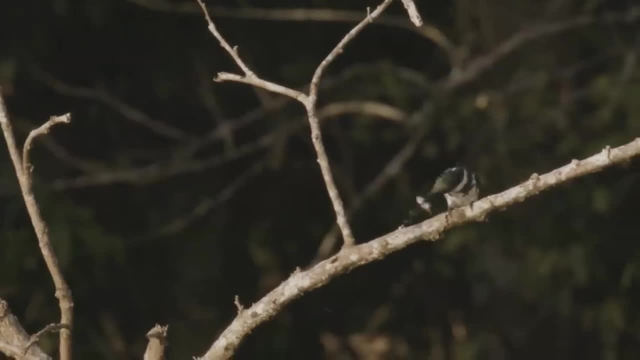 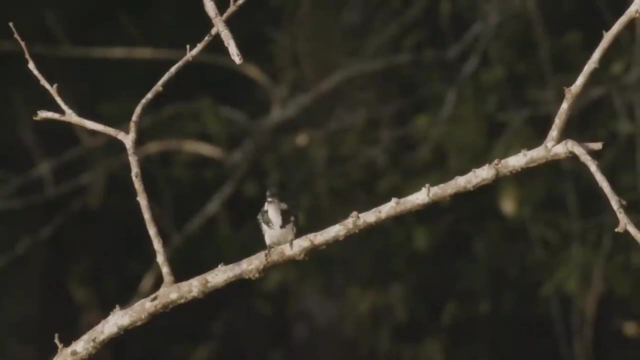 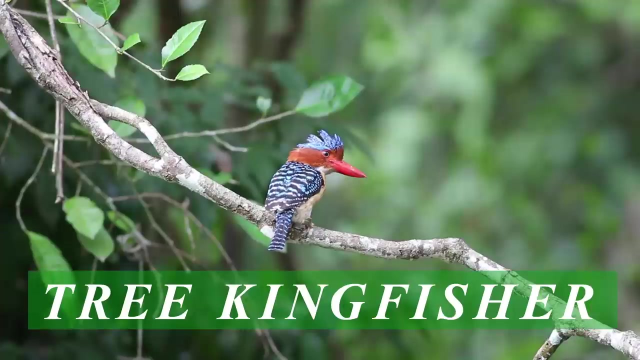 first to stun it before swooping in for the kill. Kingfishers will also smack their prey around, if it's struggling too much, before swallowing them whole. There are three subspecies of kingfisher Tree. kingfishers make up the largest subfamily and there are over 70 species, including several. 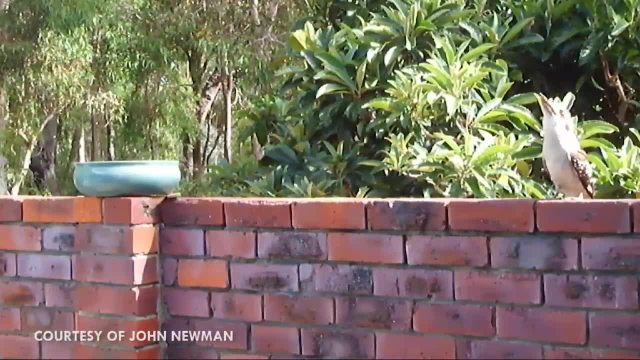 different kookaburras. Tree kingfishers are most common in the wild and they are the largest in the wild. They are the largest in the wild and they are the largest in the wild. Tree kingfishers are most common in the wild and they are the largest in the wild. Tree kingfishers are the most common in the wild and they are the largest in the wild. Tree kingfishers are the most common in the wild and they are the largest in the wild. Tree kingfishers are the largest in the world and usually only available in South America. 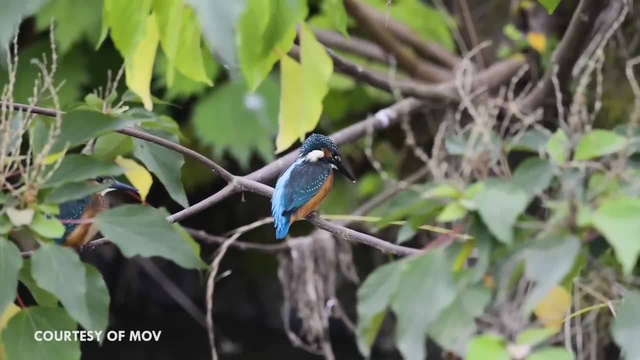 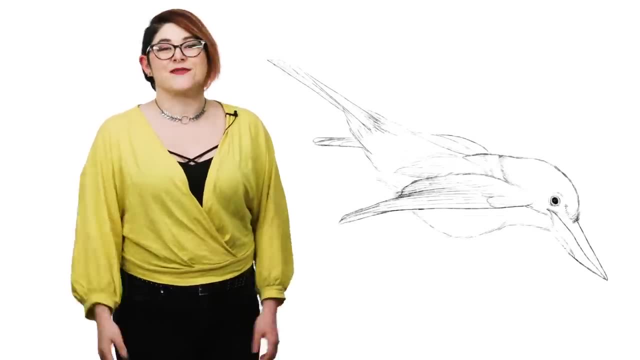 most common in Asia and Oceania and are often found in tropical rainforests and open woodlands. These kingfishers don't specialize in fish, and instead their diet is made up of the small vertebrates and invertebrates, Many species of tree kingfishers and other. kingfishers that eat primarily insects have shorter bills than their fish-eating cousins. River kingfishers are found in the old world and in Australia. As you may have guessed from their names, they are found in corporate fish specially. river kingfishers eat fish, but they'll also eat insects, Interestingly enough. 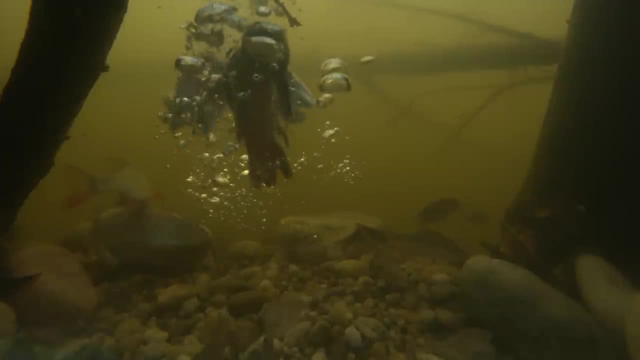 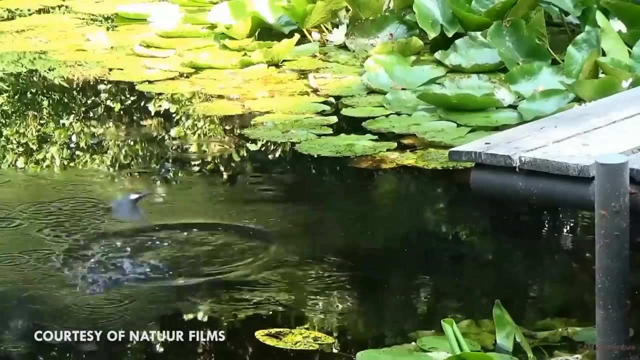 you can tell which kingfishers eat fish and which eat insects by looking at their beaks. Insectivorous species have red bills and fish eaters have black bills. Insectivorous river kingfishers can even catch flying insects in midair. 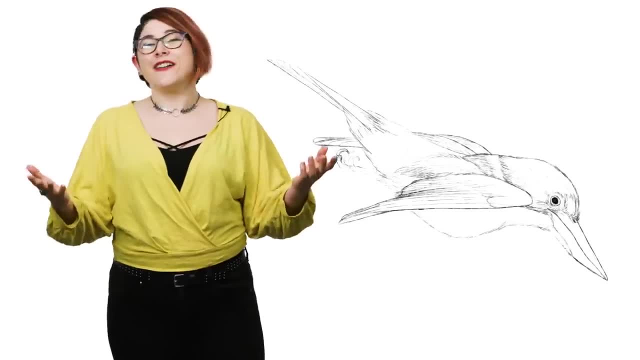 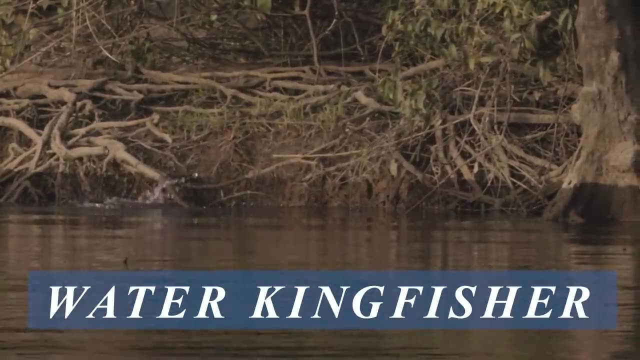 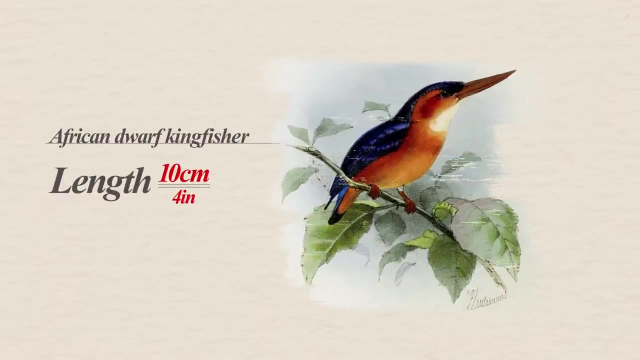 And finally, water kingfishers. This is the smallest subfamily of kingfishers, with only nine species, six of which are found in the Americas. Kingfishers vary in size, from the African dwarf, which is about 10 centimeters long, to the giant. 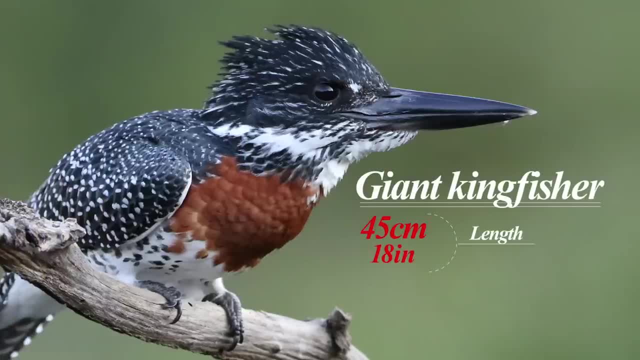 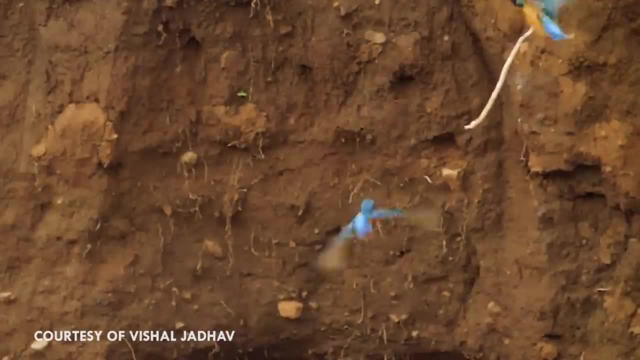 kingfisher which is about 45 centimeters long. The heaviest of the kingfishers is the laughing kookaburra, at about 500 grams. Kingfishers nest in holes, usually in tunnels in the ground. The largest known tunnel dug by a. 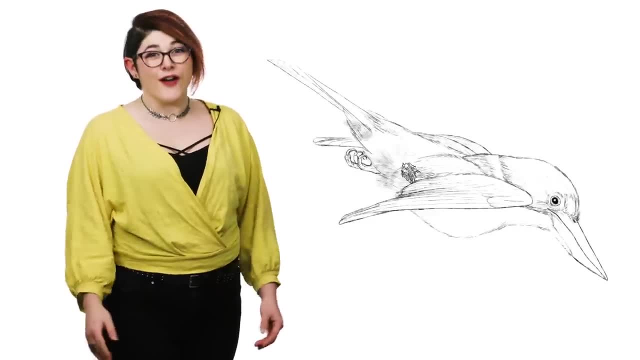 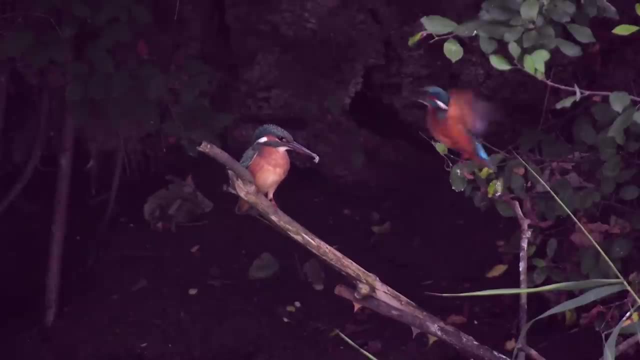 giant kingfisher was 8.5 meters long. Though there are some species of kingfisher that will live in arboreal termite nests, Most species of kingfisher are monogamous and are very territorial. They'll put up a fight for the best. 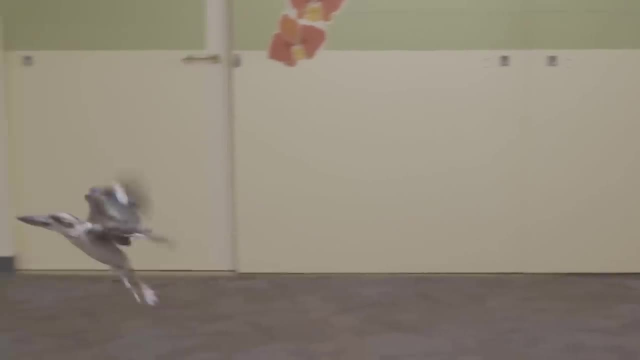 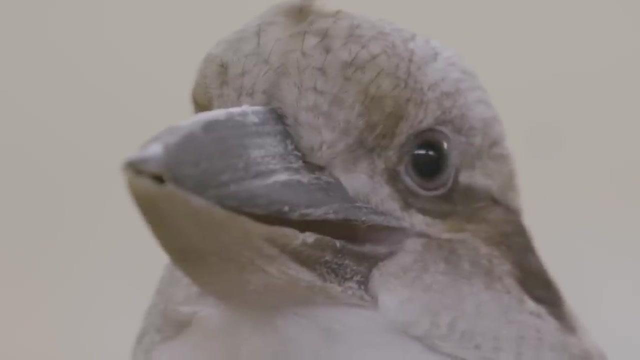 fishing spots. Laughing kookaburras, unlike many of their cousins, will stay in the same territory year round. They use their maniacal joke to run around the water, but they're not afraid to throw their or laugh to warn others to keep out. 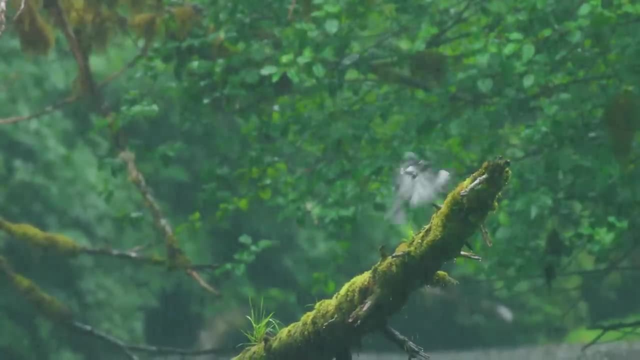 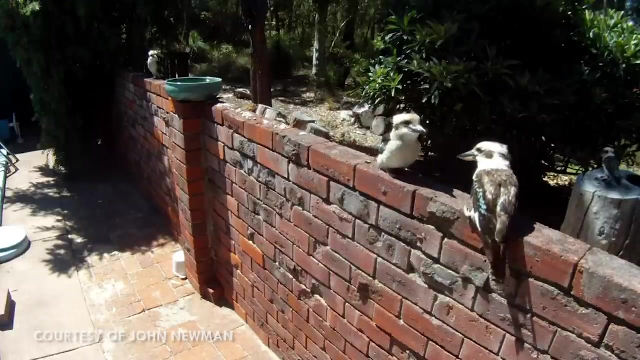 Frightening. Both parents will incubate the eggs and feed the chicks. Some species, like the laughing kookaburra, exhibit cooperative breeding and will help raise young. that is not their own, While many species of kingfisher are stable. 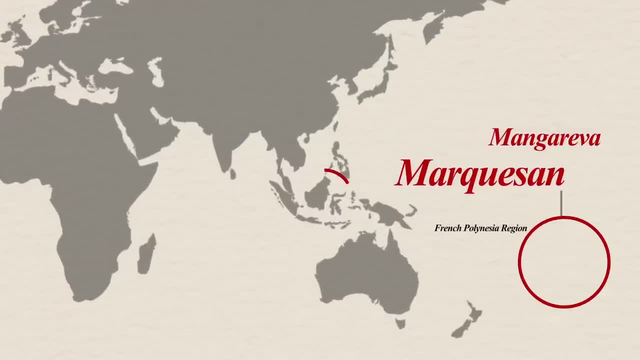 not all are so lucky. The marquesan, Javan, blue banded, mangareva and sanga dwarf kingfishers are all critically endangered, primarily due to habitat destruction. Kingfishers are some of the greatest fishers on the planet.